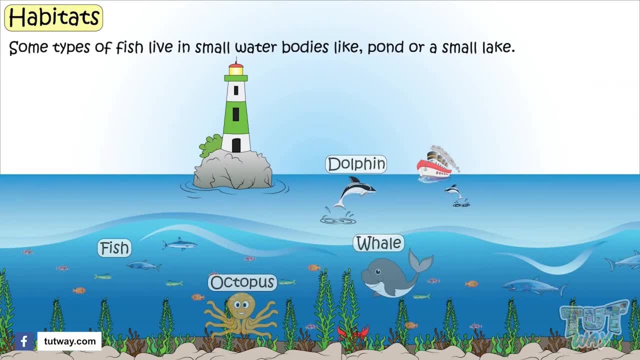 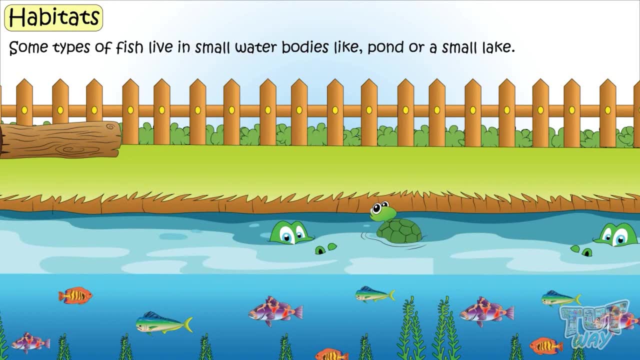 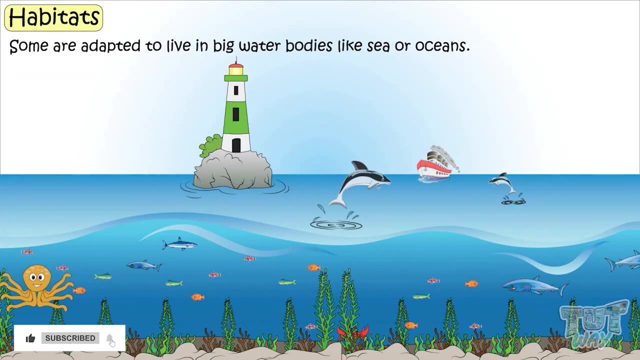 octopus. Some types of fish live in small water bodies like pond or a small lake, So pond or a lake is their habitat. Some are adapted to live in big water bodies like sea or water. Some are adapted to live in big water bodies like sea or water. 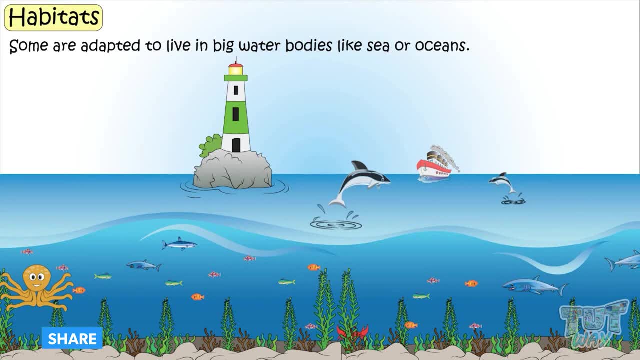 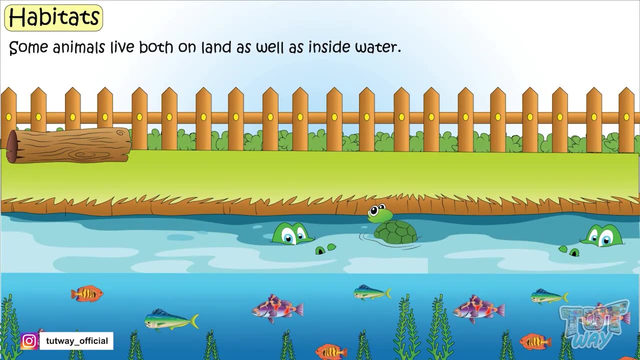 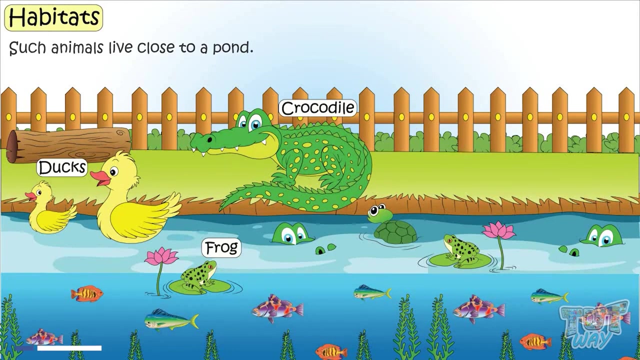 Or oceans, Then the sea or ocean is their habitat. Like whales, live in the sea or oceans only Some animals. both live on land as well as inside water, Like frogs, crocodiles, ducks. So such animals live close to a pond, So a pond and the surrounding area is their habitat. 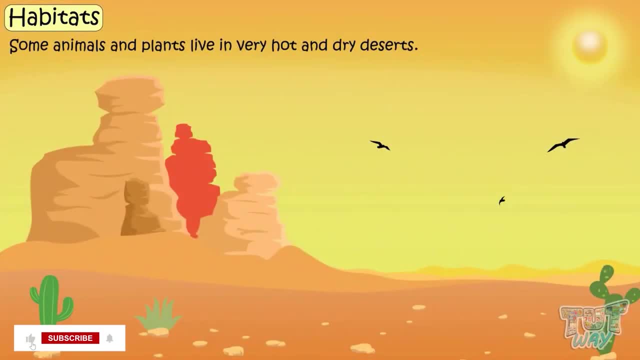 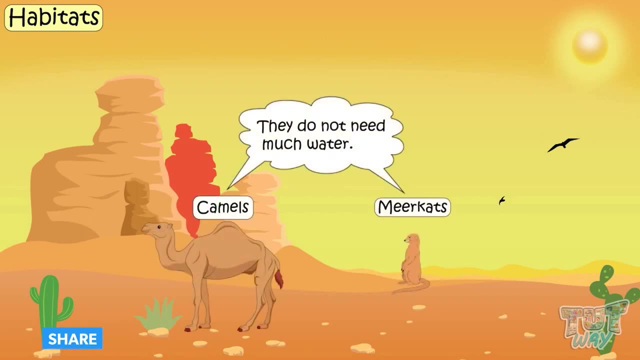 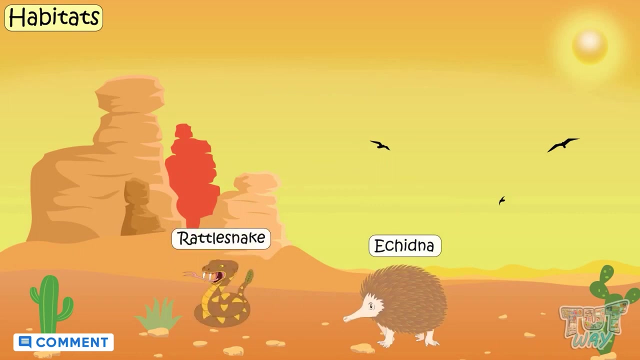 Some animals and plants live in hot and dry deserts, like camels and meerkats. They do not need much water. More examples of animals that live in deserts are enchidna rattlesnakes. They, too, live in deserts, So deserts is their habitat. Cactus is a plant that grows in deserts. 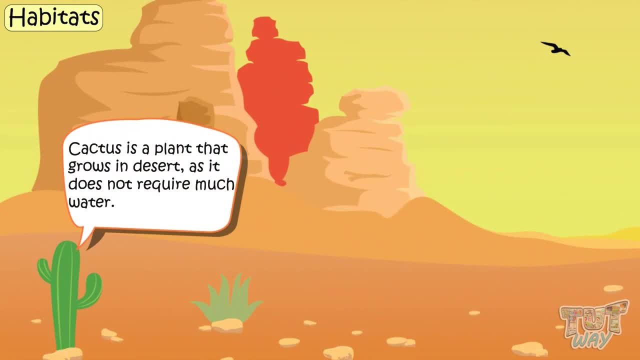 mostly As it does not live in deserts. it is a plant that does not live in deserts, So it is a require much water. so desert is a habitat for cactus plants, and desert provides them for all they need. so the most comfortable place for cactus is 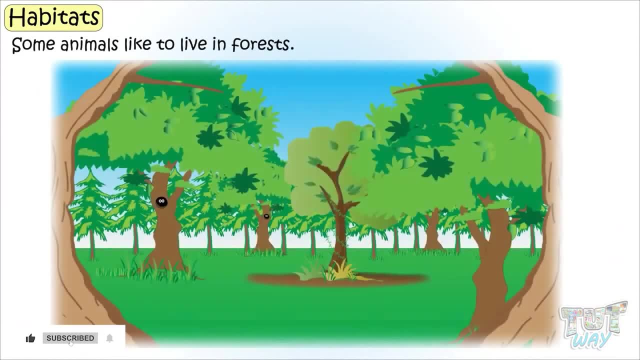 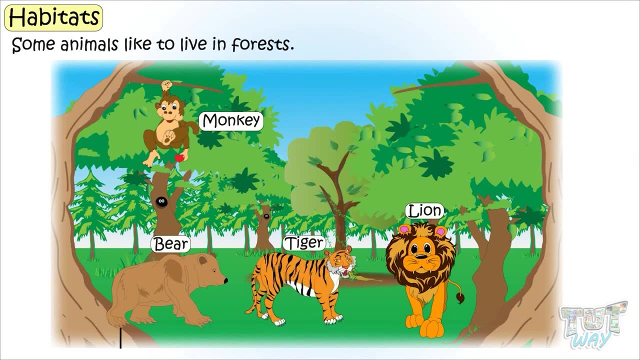 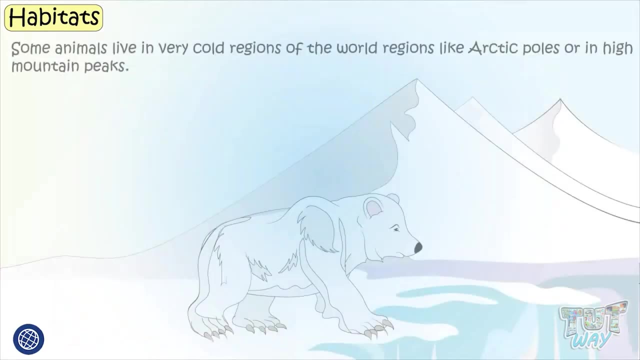 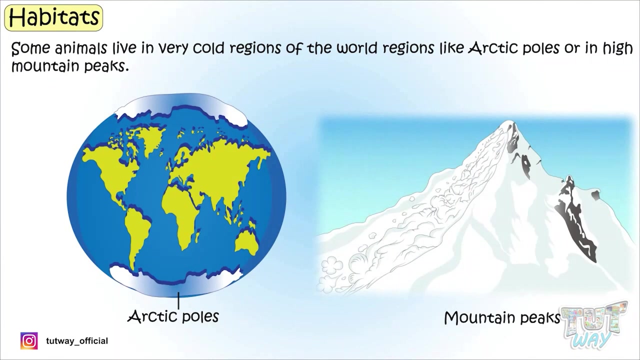 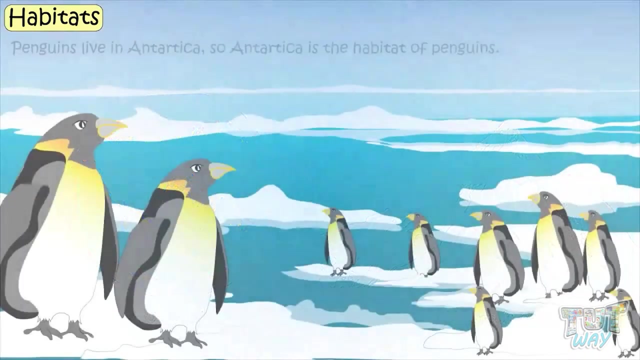 deserts. some animals like to live in the forest- monkeys, bears, lions, tigers, different types of snakes, birds- so forest is a habitat for them. some animals live in very cold regions of the world, like Arctic poles or in high mountain peaks, so they are adapted to live in very cold regions, like penguins. 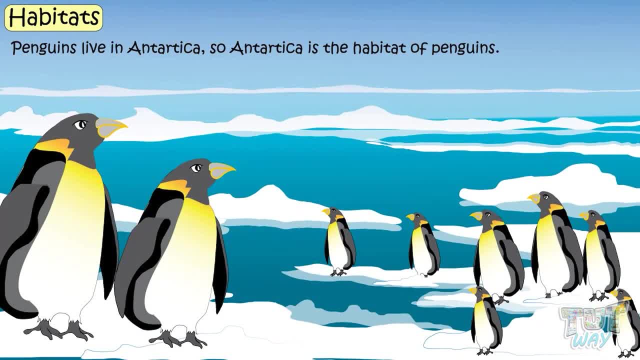 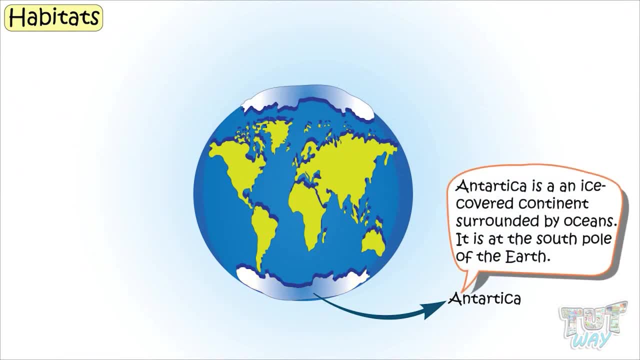 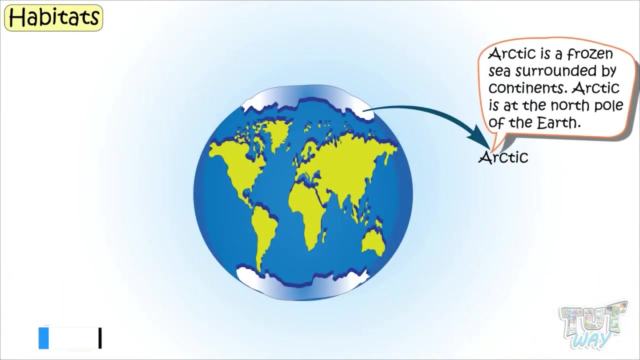 live in Antarctica, so Antarctica is a habitat of penguins. Antarctica is an ice-covered continent surrounded by oceans. Antarctica is at the south pole of the Earth- Polar bears. Polar bears live in the Arctic. The Arctic is a frozen sea surrounded by continents. 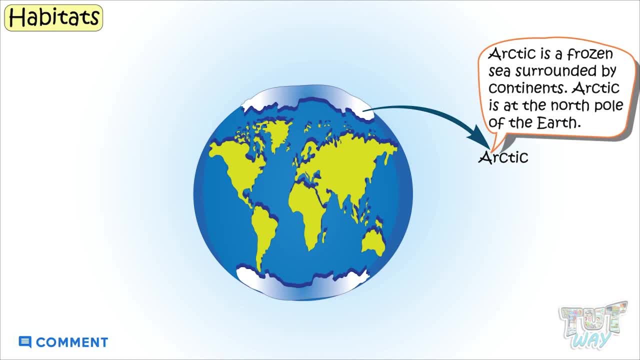 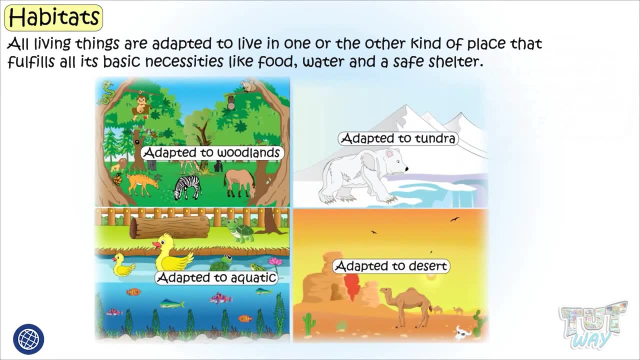 Arctic is at the north pole of the Earth, So all living things are adapted to live in one or the other kind of place to live that fulfill all its basic necessities- Food, water and a safe shelter- And that place where a species or a type of living being is most comfortable to live. 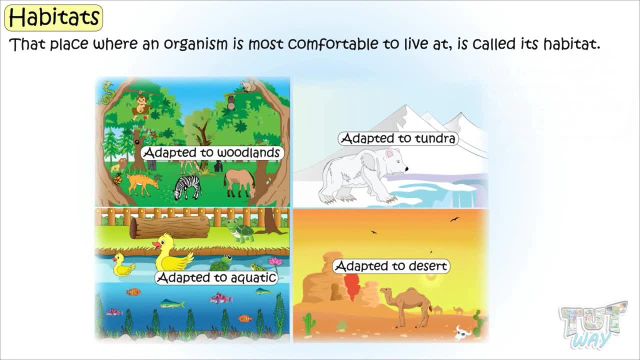 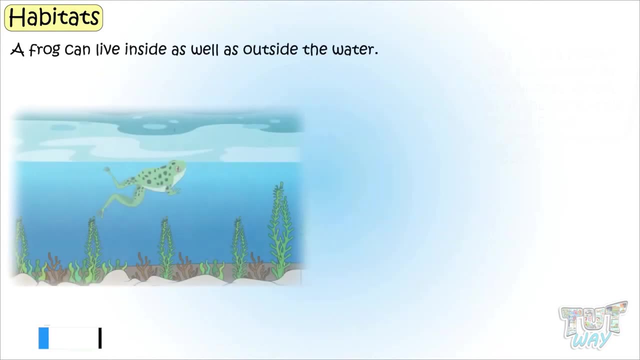 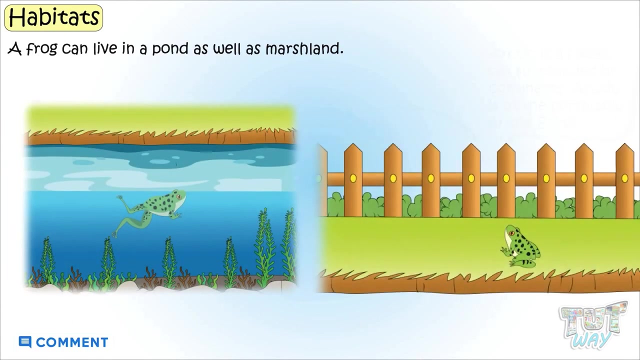 that is called its habitat, And there are different types of habitats. Most of the animals are adapted for one or two types of habitat. Like a frog, can live inside as well as outside water. A frog can live in a pond or a marshland. 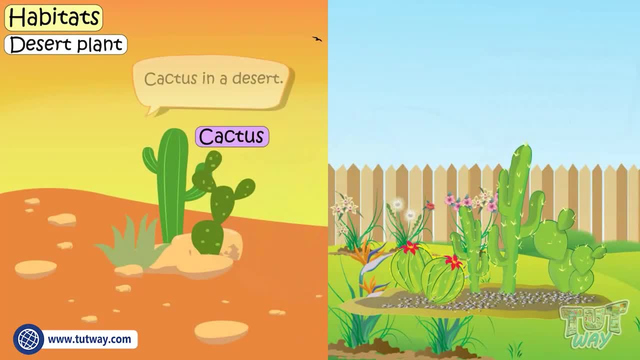 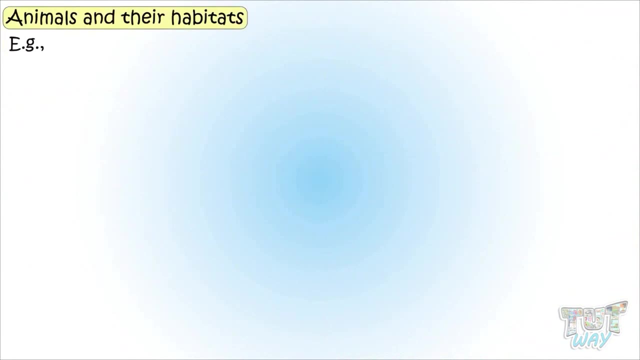 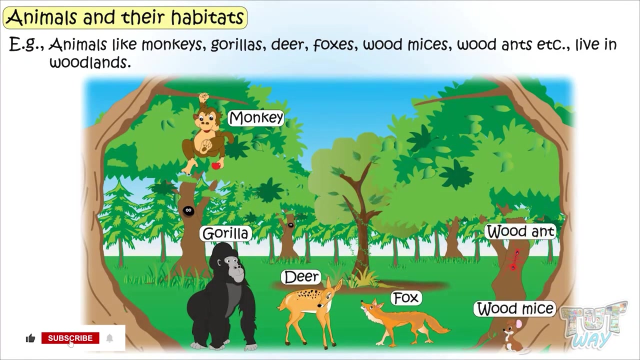 Desert plants like a cactus can grow in the desert, But can easily be grown in plain areas too. Let's see. Let's see some more examples of animals and their habitats. Animals like monkey, gorilla, deer, foxes, wood mice, wood ants live in woodlands. 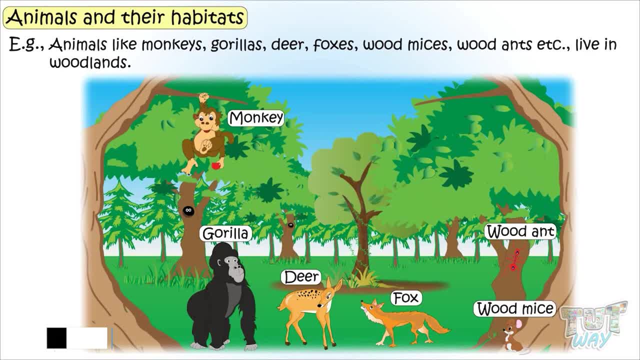 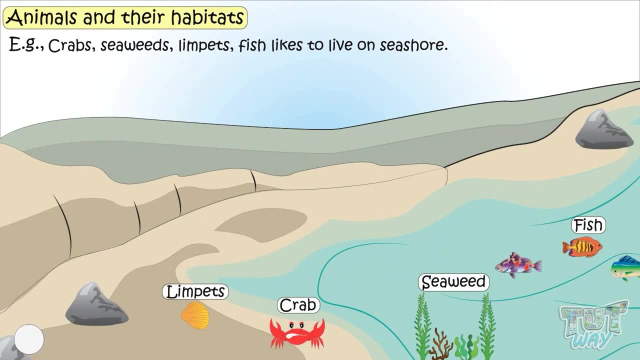 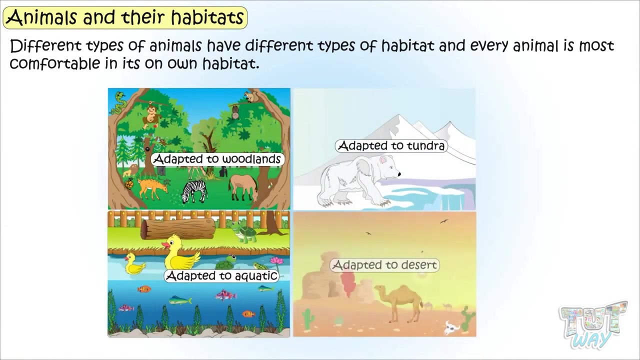 So woodland is their habitat. Crabs, seaweeds, limpets, fish like to live on seashores, So a seashore is their habitat. So different types of animals have different types of habitats, And every animal is most comfortable in its own habitat. 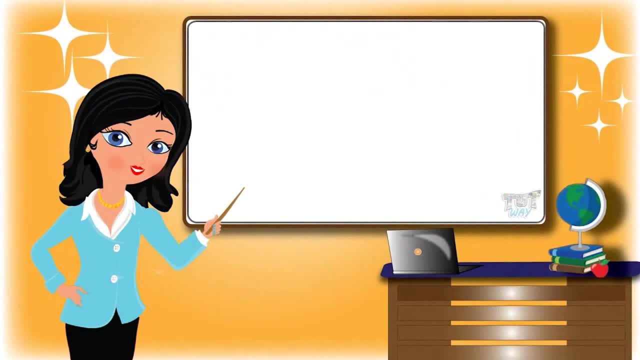 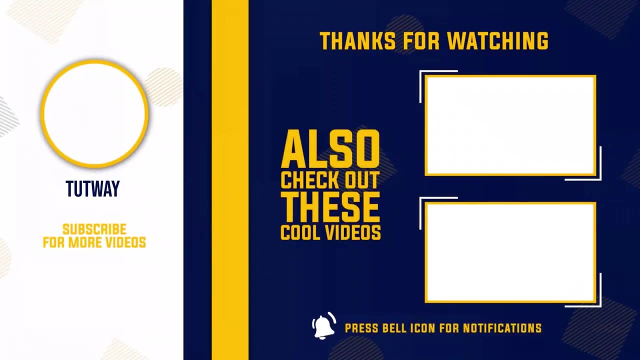 So kids now go ahead and take a quiz to learn more. Bye-bye. Thank you so much for watching. Don't forget to like, comment and share this video, And if you want to see more fun videos, you can hit that subscribe button. 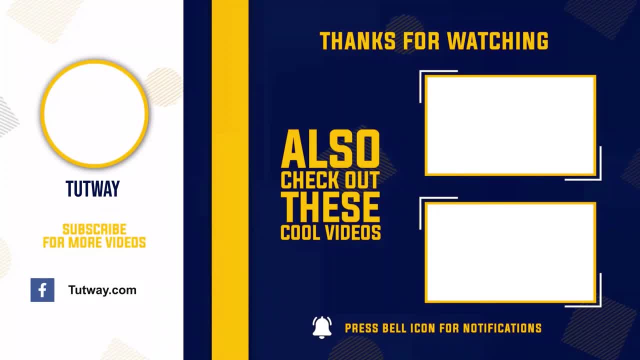 And if you want to see more fun videos, you can hit that subscribe button. And if you want to see more fun videos, you can hit that subscribe button. You can also follow us on Facebook and Instagram for more content. You can also follow us on Facebook and Instagram for more content. You can also follow us on Facebook and Instagram for more content. Bye-bye, Bye-bye.